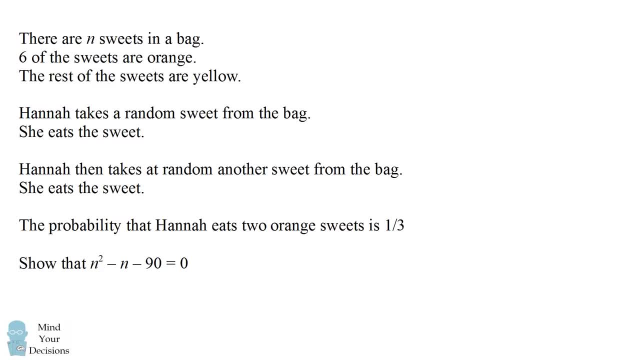 Oh my gosh. we have a quadratic equation that results from a probability problem. What does that have to do with eating sweets? This is impossible. We need to get rid of this exam. Let's sign a petition. Can you figure out this problem? 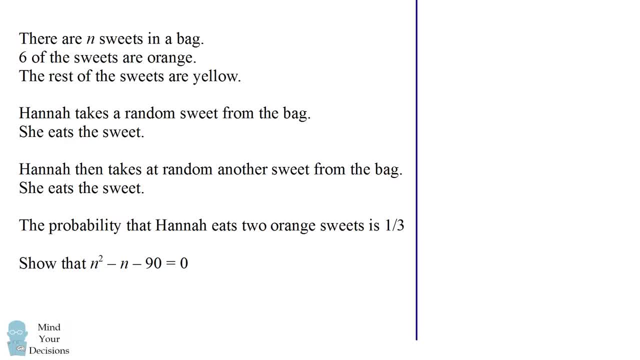 Let's work it out. Let's work through it step by step. We know that the probability that Hannah eats two orange sweets is one-third. We'll write that as a statement: that the probability of two orange sweets is one-third. That means the first and second draws are equal to one-third. 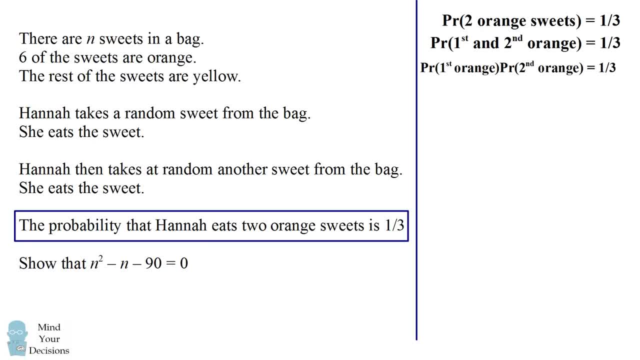 and that means the probability of the first draw times. the probability of the second, conditional on the first, is also equal to one-third. Now we need to figure out what the probability of the first draw is. We need to figure out what the probability of the second. 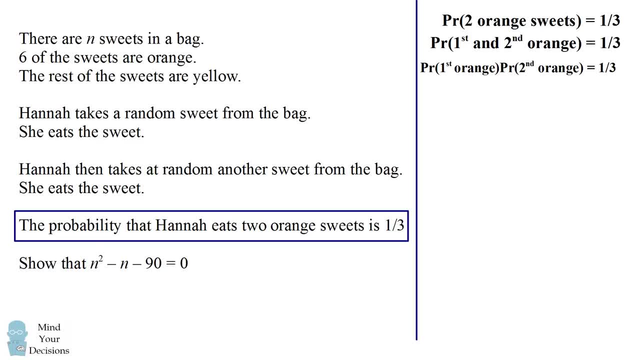 draw is The probability of the first draw being orange and the probability of the second draw being orange conditional on the first draw being orange. So let's work out the probability. the first draw is orange. This is the number of orange sweets divided by the total number of sweets in the 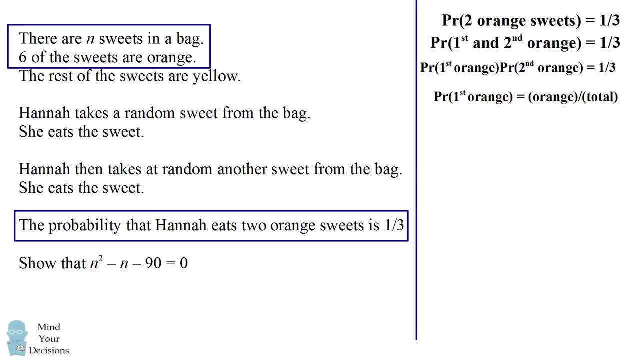 bag. There are six orange sweets and there are N sweets in the bag. We don't know what N is. N is a variable, but the total number is equal to N, So we can write this. The probability that she draws another orange sweet is a little trickier. We need to take into 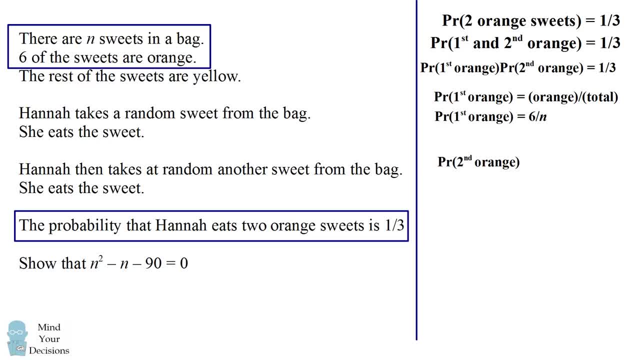 account. she's already removed one orange sweet from the bag, So there will be one fewer orange sweet and there will be one fewer sweet in total. You can think about this like drawing cards from a deck: If you draw an ace from the deck, what remains in the deck will have. 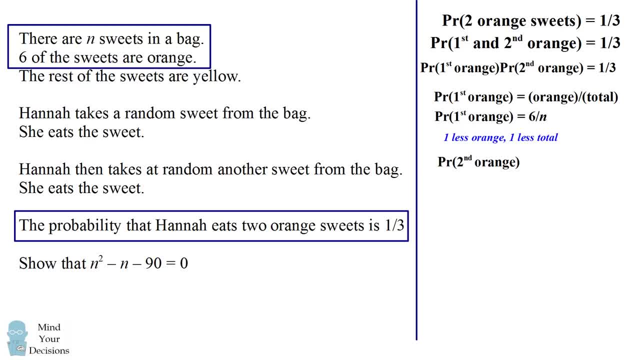 one orange sweet. So if you draw an ace from the deck, what remains in the deck will have one fewer ace and one fewer card. So we have one fewer orange sweet, which is five, and we have one fewer candies in total, which means N minus one. So the conditional probability of drawing the 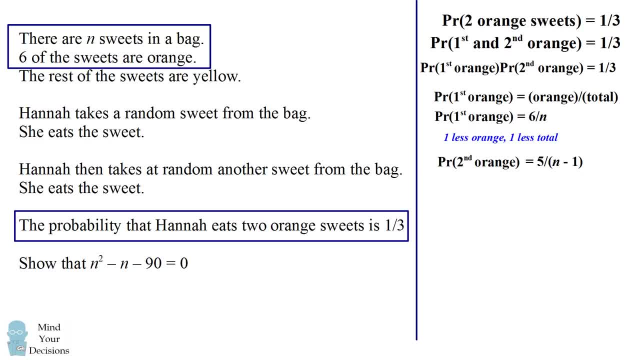 second sweet as orange, is five divided by N minus one. We go back to our equation that the probability that she drew two sweets in a row was one third. We multiply these together, Then we rearrange and simplify, So we have one fewer ace and one fewer card. So we have one fewer orange sweet, which is: 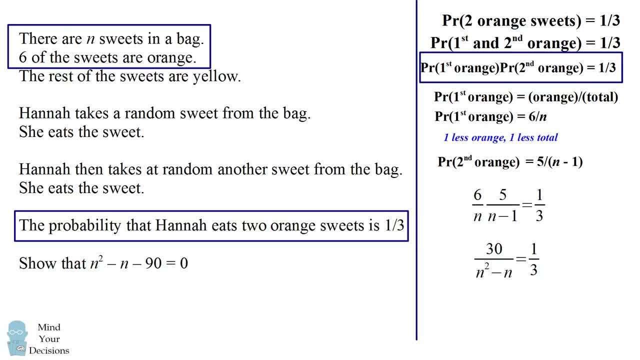 five. So we get 30 divided by N squared minus N equals one third. Then we cross, multiply So 90 is equal to N squared minus N, And then we rearrange So we have N squared minus N minus 90 is equal to zero. That's what the first part of the problem wanted you to prove, And it's kind. 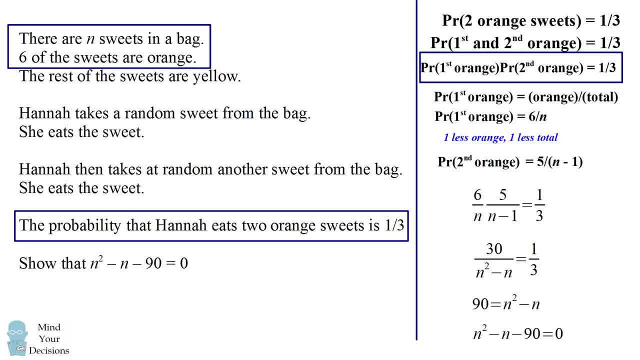 of interesting. You can get to this level without knowing how many sweets there are in the bag. What if you didn't know all this? What if you just said: all right, N squared minus N minus 90 equals zero. Let's say we wanted to check our work, that this: 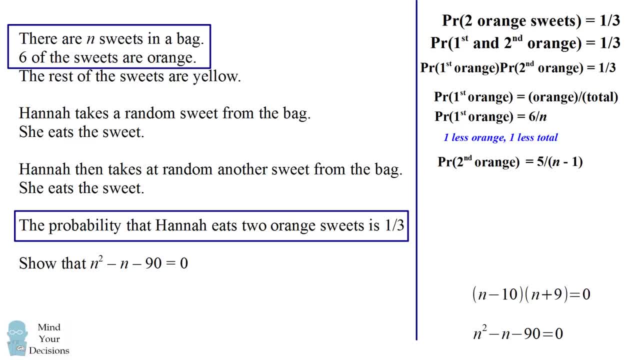 actually works. So we factor this into N minus 10 times N plus nine equals zero, which means N is either equal to 10 or minus nine. We can't have minus nine because the number of candies in the bag should be a positive number, So we have N equals 10.. So let's check if this actually 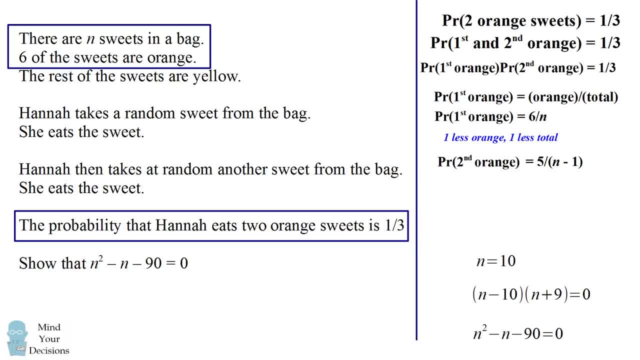 works out, If she draws an orange sweet on the first draw, that'll be six over 10.. And then the second draw will be five over nine. Multiplying these together we do in fact get one thirds. So there are 10 sweets in the bag, of which six are orange. And in those conditions, 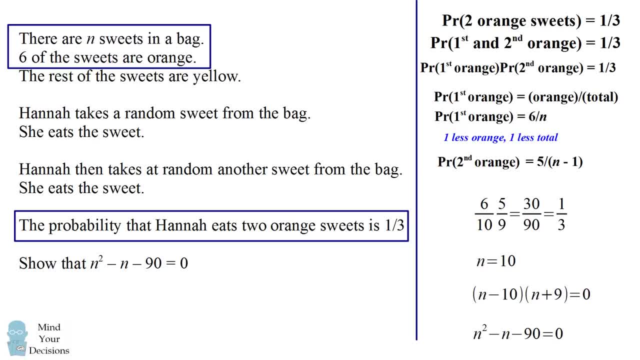 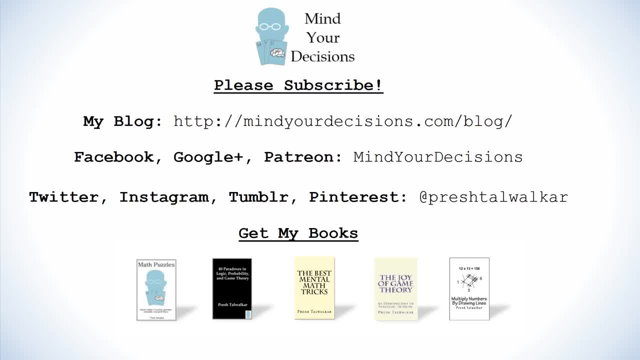 Hannah would draw two orange sweets in a row, one out of every three times. I hope you liked this video. Please subscribe to my channel. I make videos on math, math and game theory. You can catch me on my blog, Mind Your Decisions, where I cover problems like 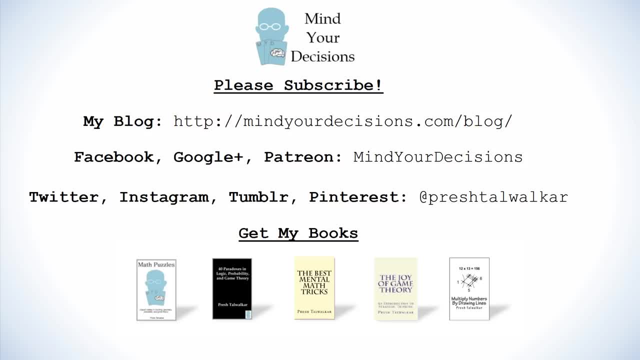 this every single week in a Monday puzzle or Sunday puzzle. You can also follow my blog on Facebook, Google Plus and Patreon. You can catch me at Presh Talwalkar on a bunch of social media sites And check out my books. I write a bunch of books about math. If you read my books about 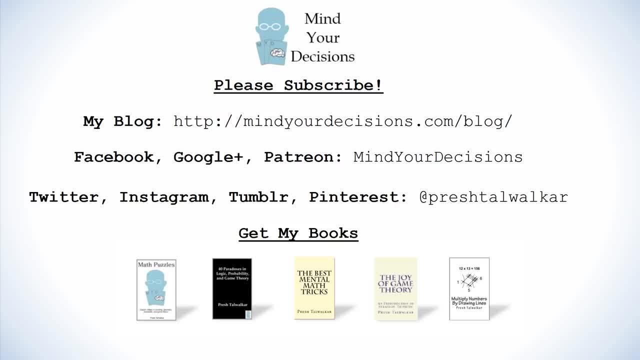 math puzzles, you would have been able to solve this problem in a cinch. Thanks for watching.